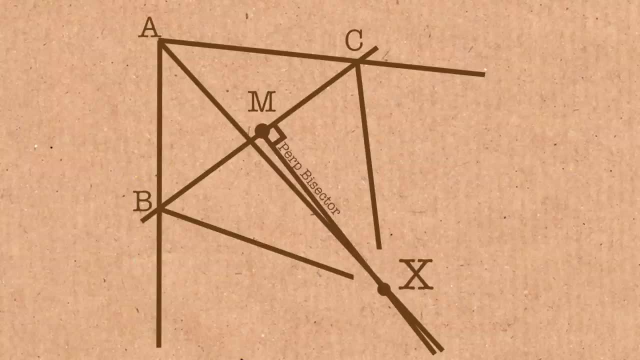 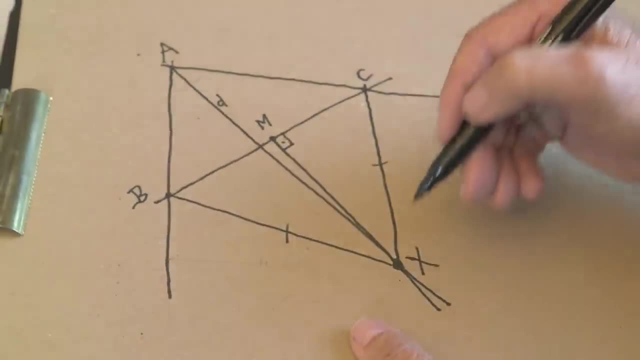 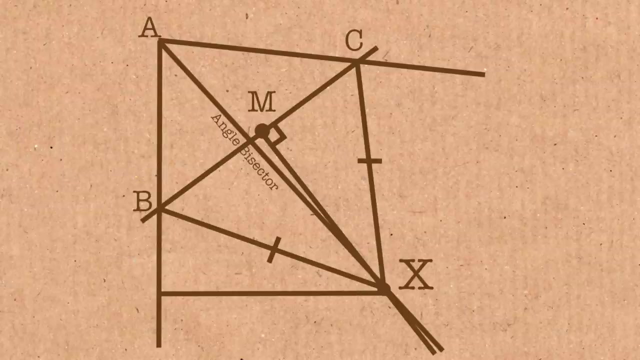 So let's draw these two lines- and we know that these are equal because they're on the perpendicular bisector- Okay, but also if I draw the shortest distance from X to line A B, which might look something like that and comes in, of course, at the right angle here, 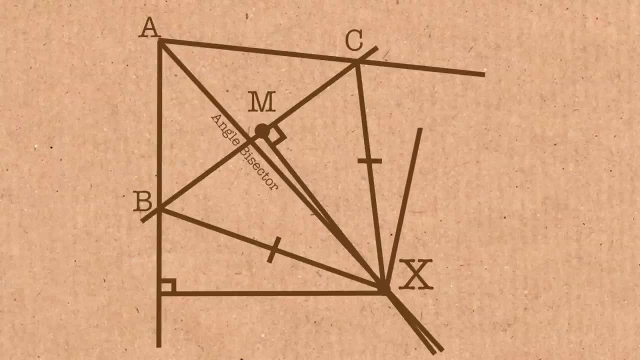 and I draw the shortest distance from X onto line A, C and at the right angle. here. let's call this point B star And let's call this point C star. Then I know that X B star is equal to X C star because we're on the angle bisector. 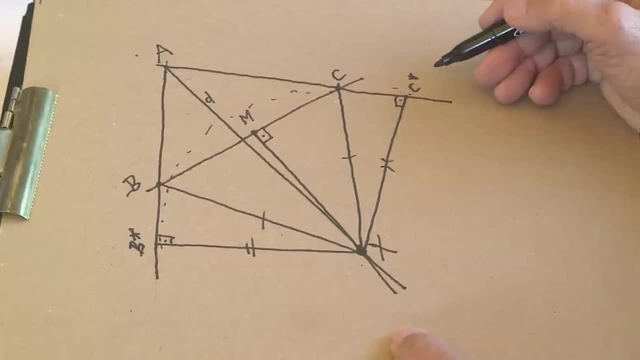 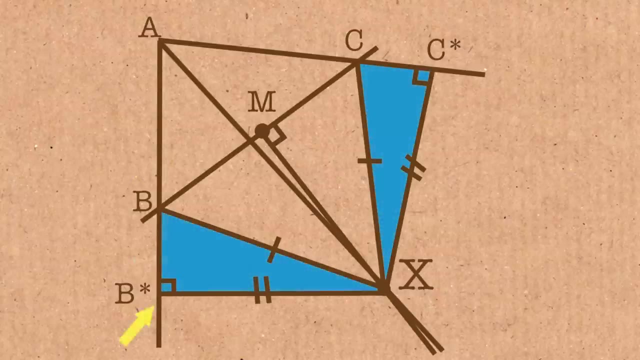 and these are all the points that are equidistant from those two lines. Okay, now we focus on these two small triangles, And here we have a triangle with a right angle. Adjacent to the right angle, we have this double-marked line X, B star. 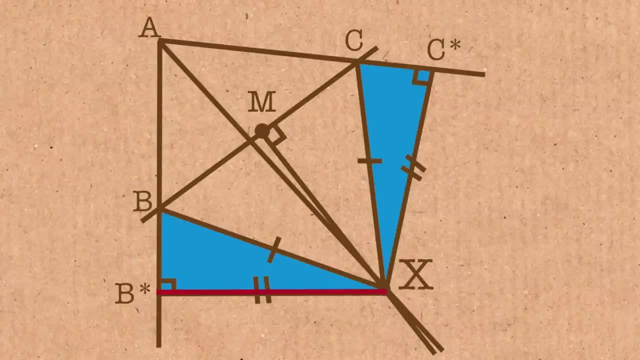 And here we have a right angle and adjacent to the right angle we have this double-marked line X, C star, And we know these two lines are the same length. We also have the third side of the triangle, which is opposite of the right angle. 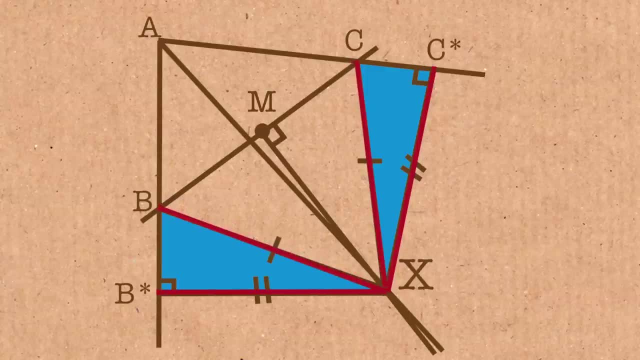 marked with this one slash and it's the same as this slash over here. That's the hypotenuse in this case. And so because two triangles, then they have two equal sides and they have the longer side being opposite to an angle that also happens to be equal. 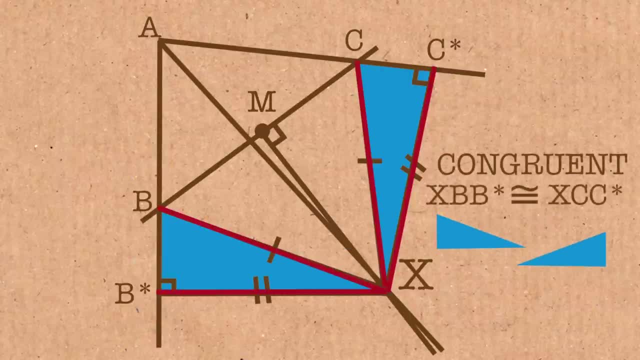 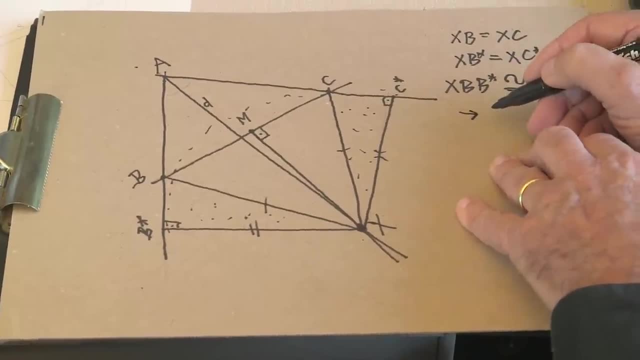 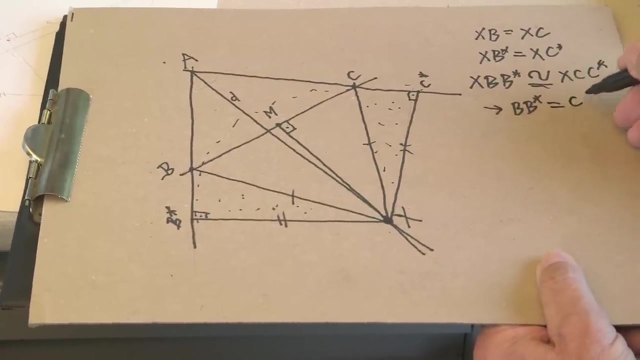 then these two triangles are congruent As a matter of fact. in this case, you can see, they're basically mirror images of one another. Now, this, of course, tells us that we also now know that B, B star then must be equal to C, C star. 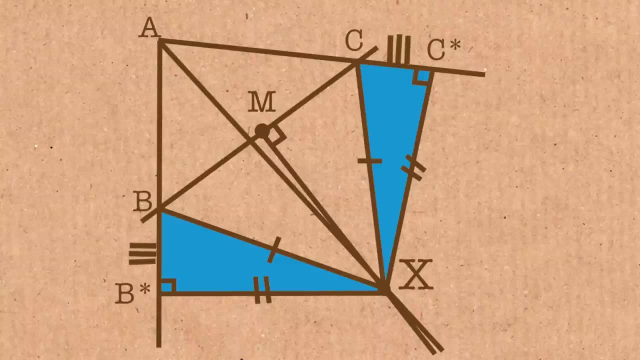 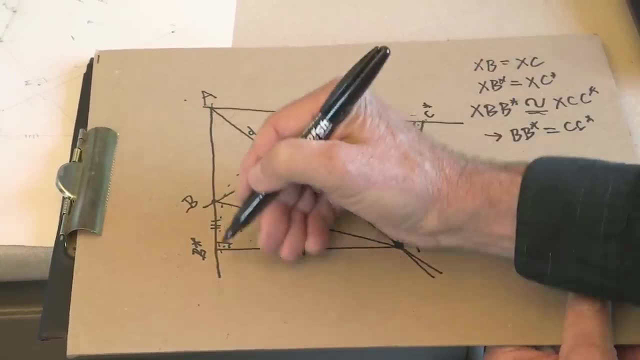 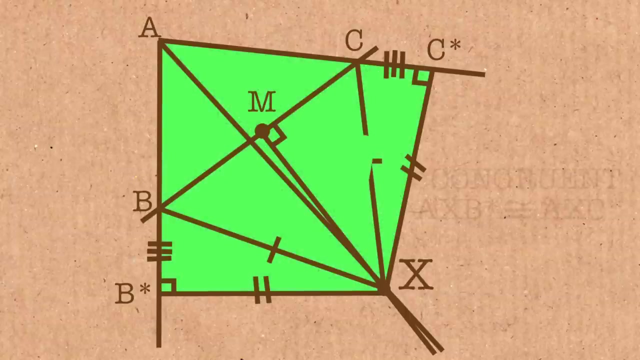 B, B star. mark it with three slashes equal to C- C star. Now we have more congruent triangles. We also have the triangle A X B star being a mirror image of A X C star, and so those two triangles are congruent. 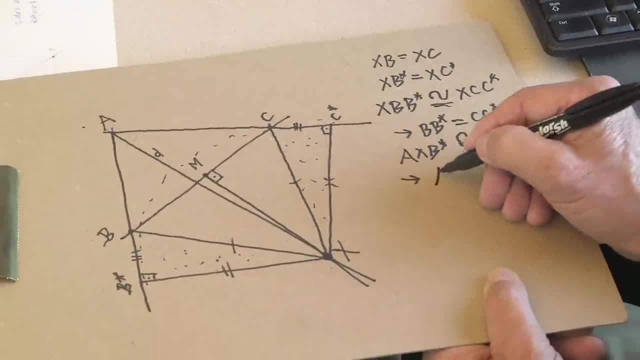 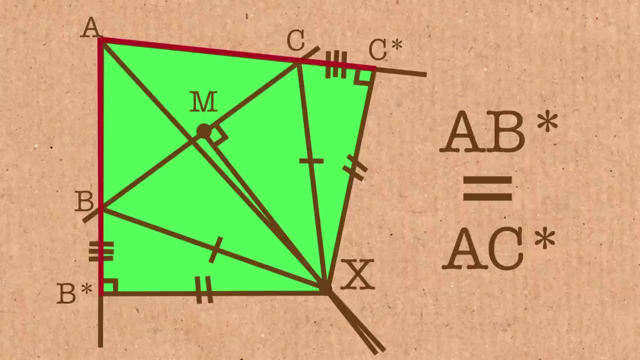 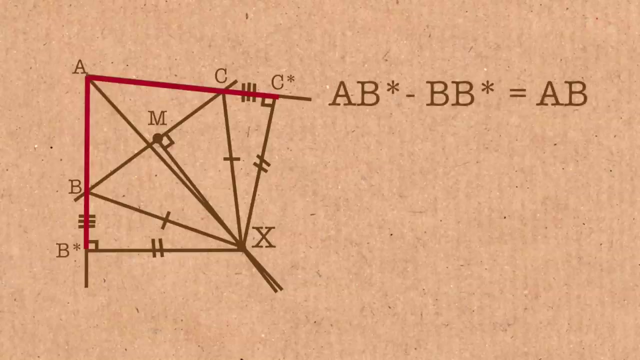 And this, of course, tells us that A B star equals to A C star. Ok, now, what can we conclude from all that? Well, we can say that A B star minus B B star is really just the side AB.